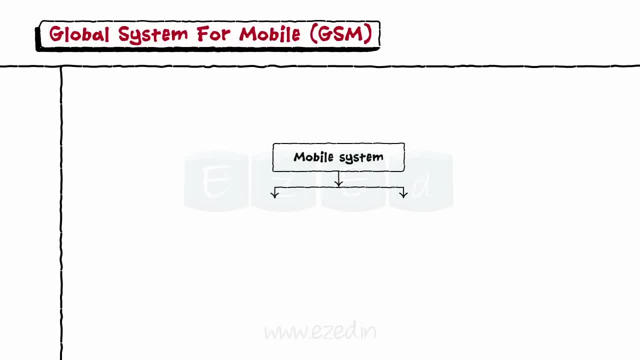 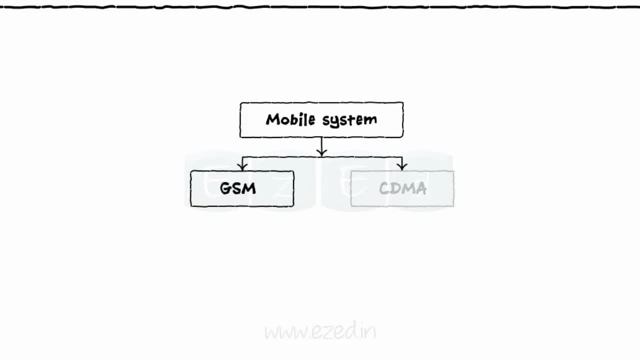 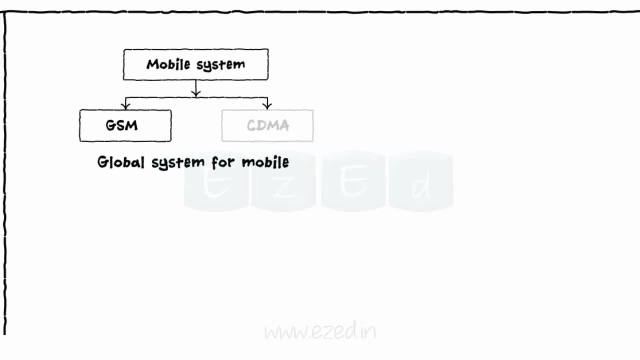 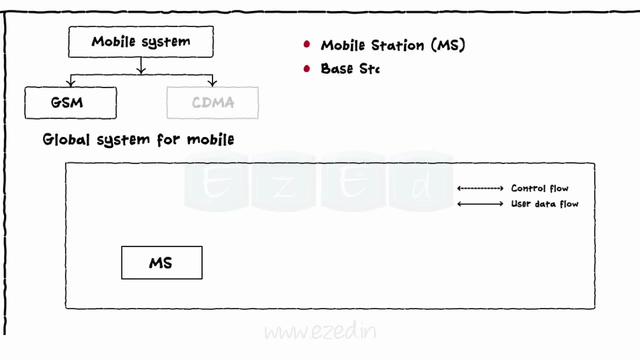 We all know that there are two types of systems available as GSM and CDMA. We will only study the basics of GSM system. GSM stands for Global System for Mobile. GSM is nothing but a big system made up of few small systems such as Mobile Stations, MS, Pays Station, Subsystem, BSS. 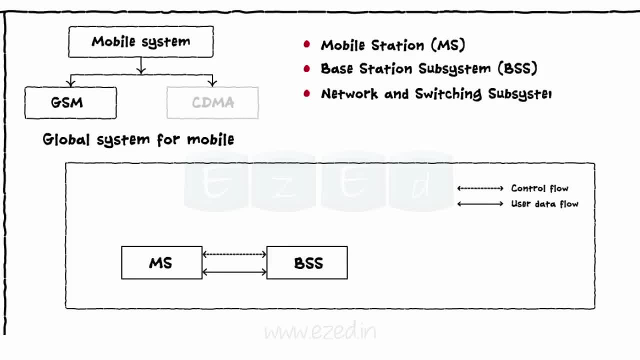 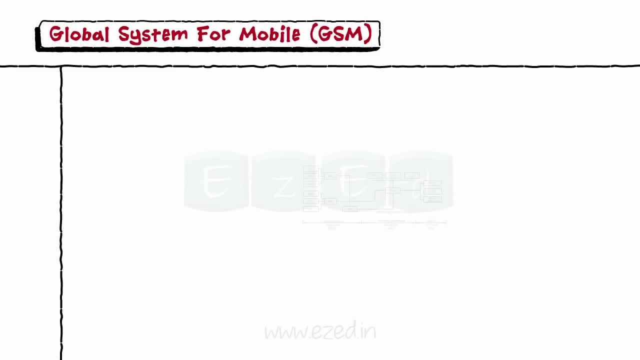 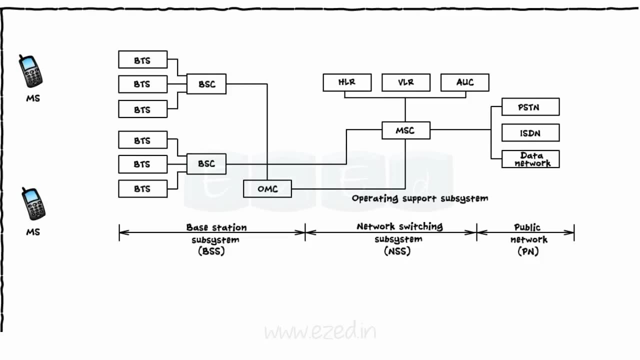 Network and Switching Subsystem: NSS. Operating Subsystems: OSS. The architecture of this GSM network is, as shown, Mobile Station MS. MS is nothing but the device used for communication, such as cell phone, fax machine, etc. Pays Station Subsystem: BSS. 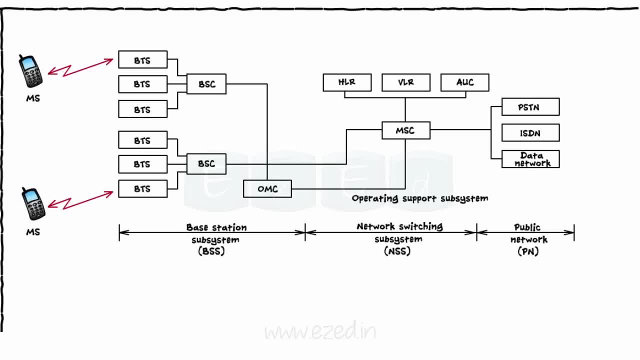 BSS gets connected to MS via radio interface. It has two different blocks as BTS Bays Transceiver System and BSC Bays Station Controller. Practically every MS gets connected to BTS of that area. This BTS sends the signal to BSC. 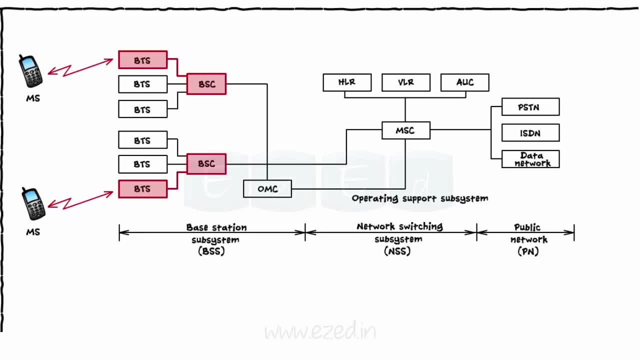 Many BTS are connected to one BSC and at the end of this, BSC is connected to MSC Hence. BSC is connected to MSC Hence. BSS system consists of BTS and BSC Network and Switching Subsystem NSS. 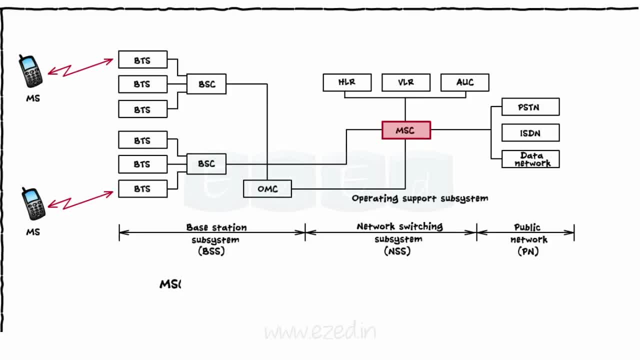 This system mainly contains MSC. MSC is the backbone of the entire network. It controls all the operations, from setting up a call till the hand-off procedure. Other blocks of NSS are HLR, Home Location Register, which keeps the database of all the users. 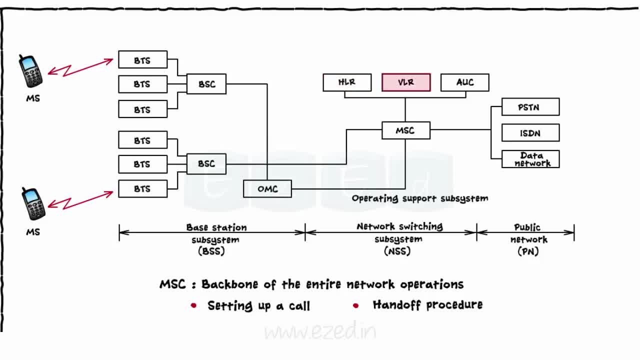 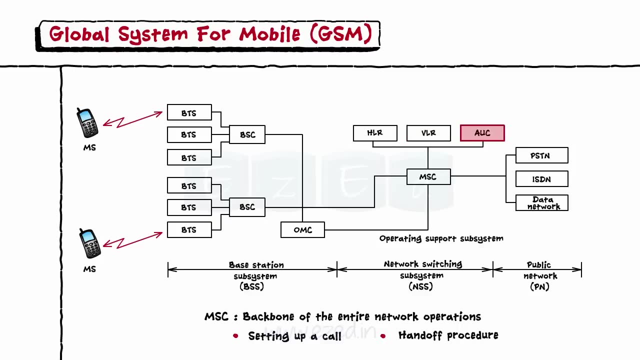 Who reside in the same geographical area. VLR Visitor Location Register Keeps the track of all the users who are visitors for that particular geographical area, Mainly roaming customers. AUC Authentication Center Mainly controls the authentication of the users by checking their SIM numbers etc. 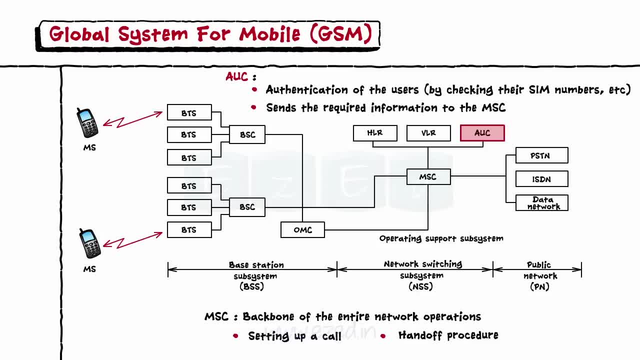 And sends the required information to the MSC. mínimastelefonecom. Thank you For thelike. nouveau usted su base can every, as with ti hago em envio dan.